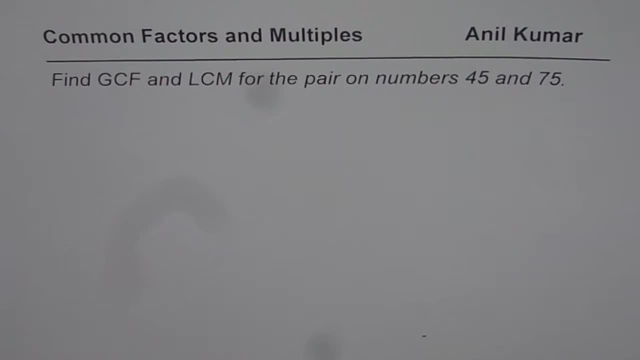 I am Anil Kumar and in this video I am going to discuss with you how to find common factors and multiples of different numbers. Question is: find greatest common factor and least common multiple for the pair of numbers 45 and 75.. We will use the method of prime factorization. 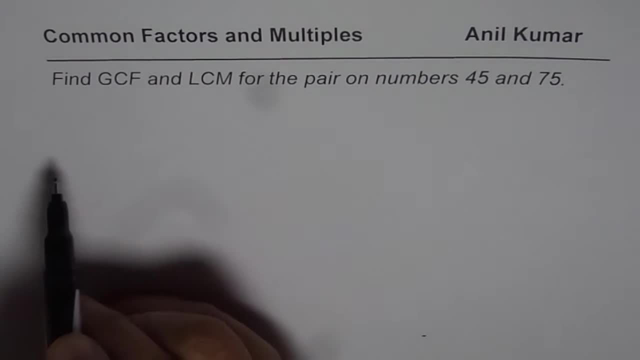 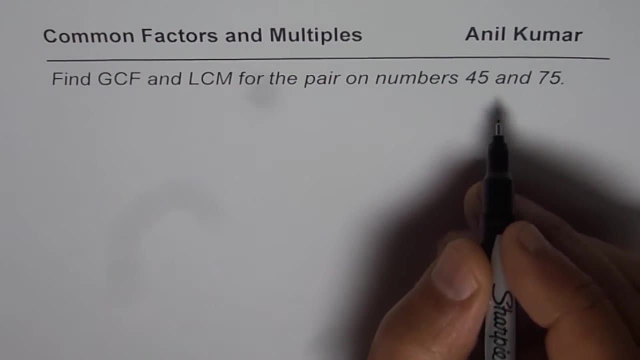 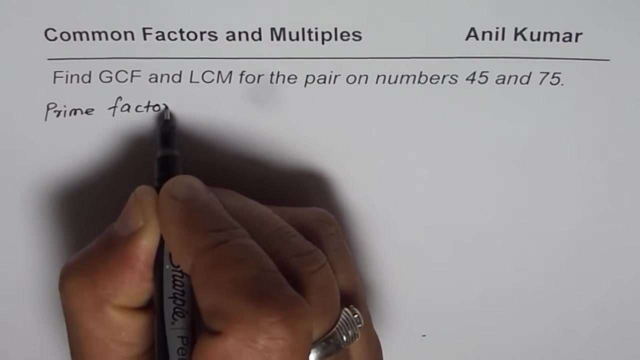 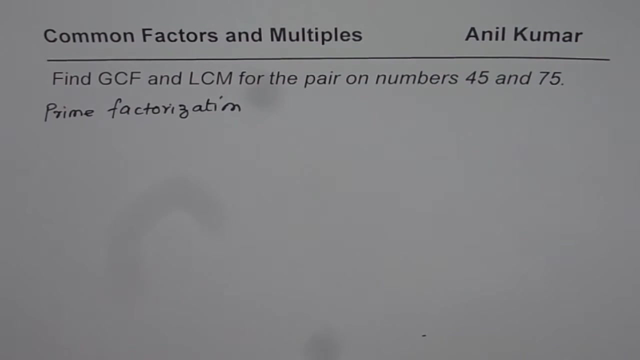 to find GCF, the greatest common factor, and LCM the least common multiple. Let us do prime factorization first. So let us do prime factorization And once we have the prime factors we will see how to find greatest common factor and least common multiple. So 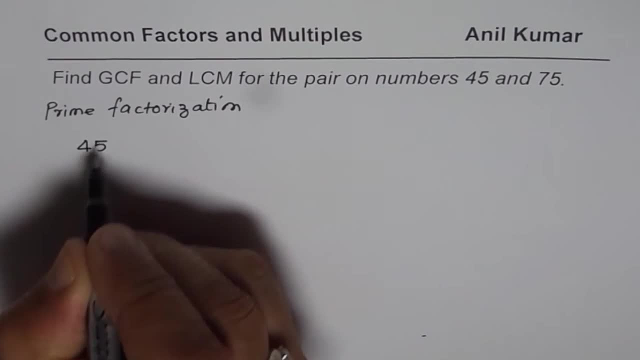 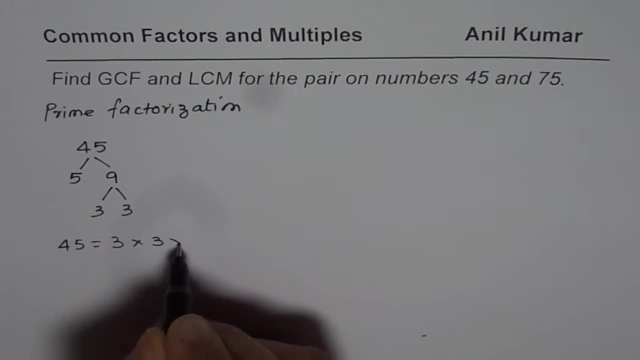 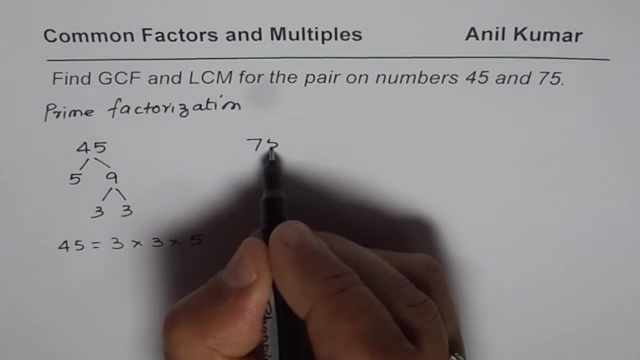 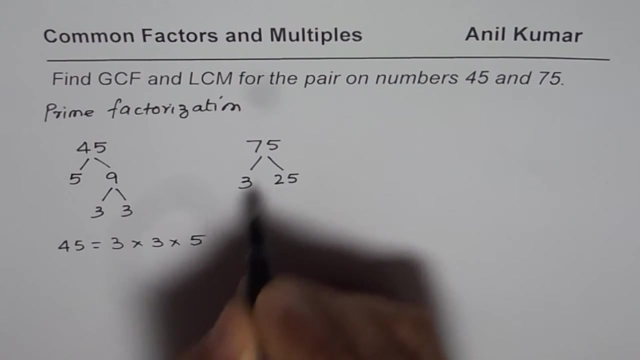 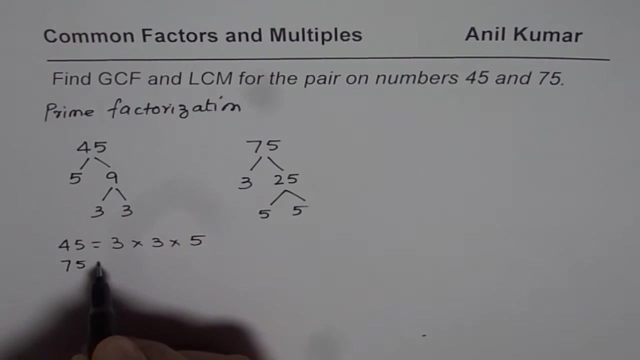 equals to 3 times 3 times 5.. Now let us factorize prime, factorize 75.. 75,, you know, can be divided by 3. So 3 times 25.. 5 is 75 and 25 is 5 times 5.. So for 75, we could write prime factors as 3,, 5 and 5.. Now let us first. 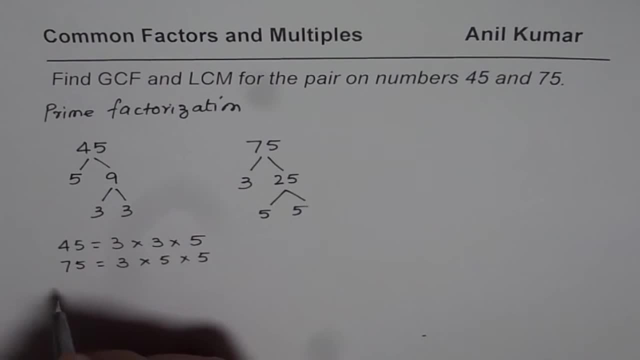 find the greatest common factor. Now, how do we find greatest common factor? This is what we learn First. let us circle around and find the greatest common factor. Now, how do we find greatest common factor? So we have 3 and 3 as the common factors. We also have 5 and 5 as the common factor. So 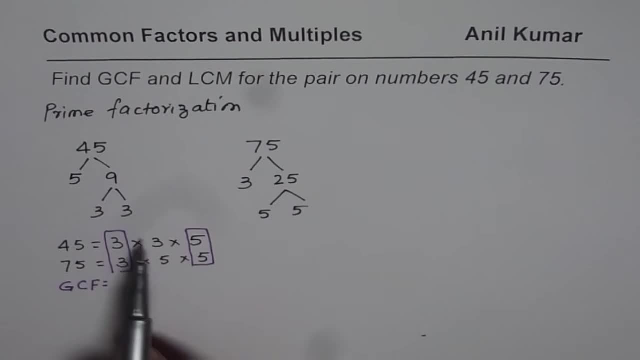 the greatest common factor is product of common factors. So greatest common factor is product of common factors. So we'll multiple 3 and 5. So 3 times 5 when you do is 15.. So that becomes common factor. Now let us see how to find least common multiple. Now least common. 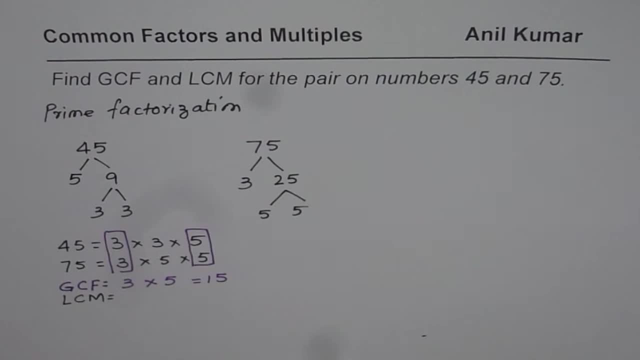 multiple is more than greatest common factor. So to find least common multiple, what we do is we have already taken care of these factors. so we start with greatest common factor and multiply by remaining factors. You get the point. So in our case the remaining factors are 3 and 5, so it will multiply the greatest. 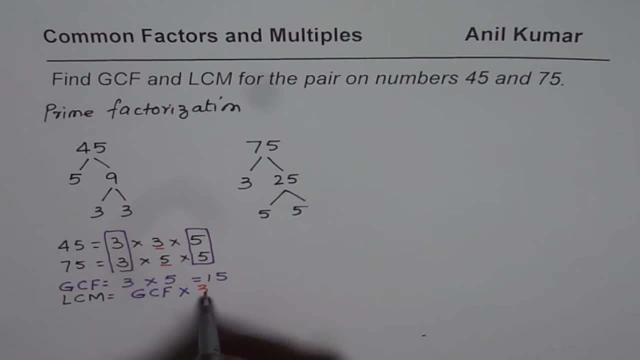 common factor by 3 and 5. so we'll multiply this by 3 and 5,, do you see that? And then we get our result, which will be the answer. So greatest common factor is 15, so we'll do 15 times 3 times 5, and that is let's use the calculator, right? 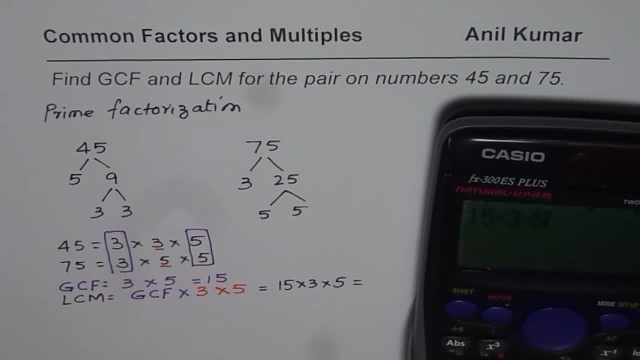 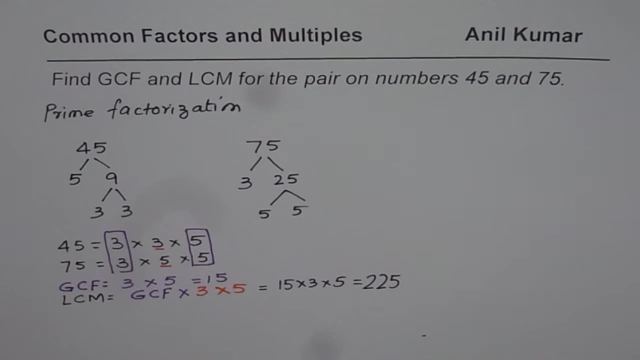 so it is 15 times 3 times 5, 2 times 3 times 5, 225.. So in this particular case, 225 is the least common multiple right. So that is the way you can find greatest common factor and the least common multiple right. So let's look into this. 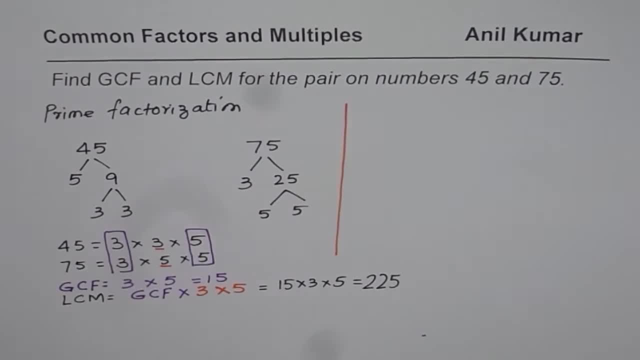 process once again and understand right. So first is we found greatest common factor. So greatest common factor is basically a number which can divide into both, the greatest number which can divide into both. How did we find that? We found that as product of 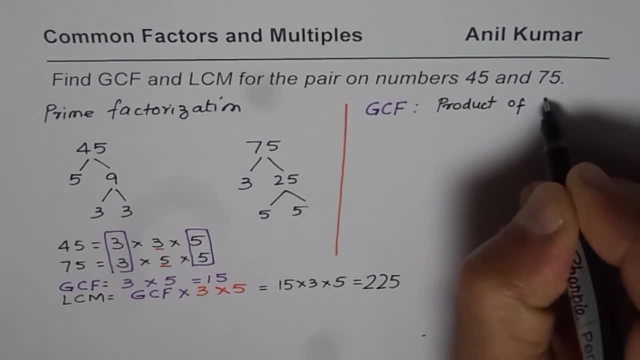 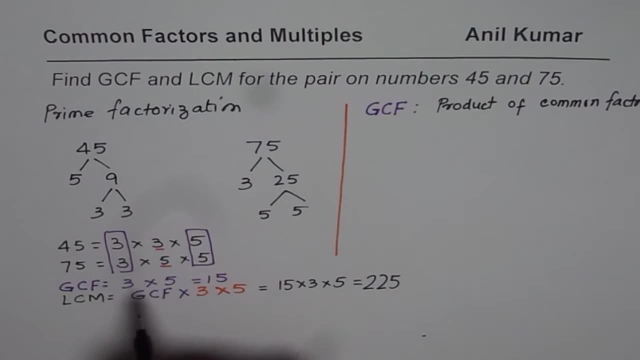 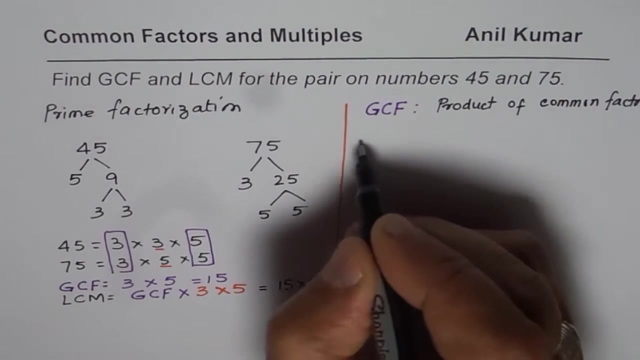 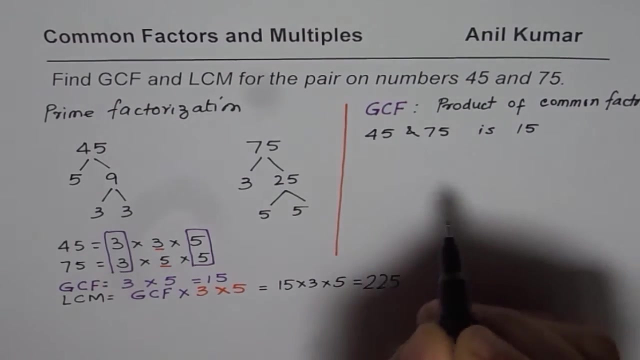 common factors. Do you see that? Product of common factors? So in our case we found greatest common factor is 15.. Right, So in our case it was so: the greatest common factor between 45 and 75 is 15.. So you can. 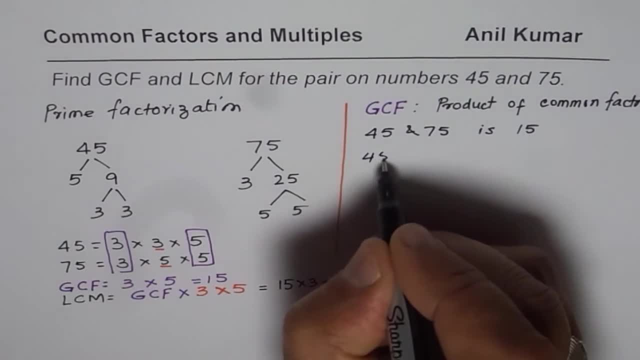 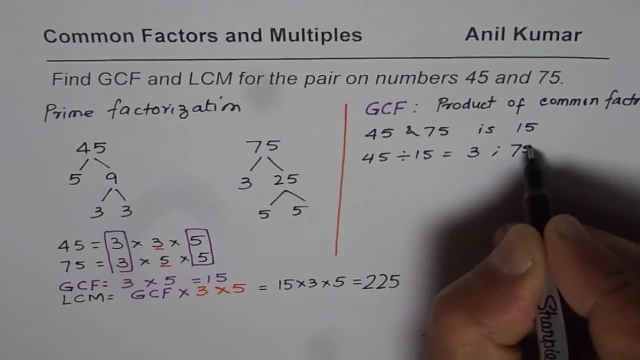 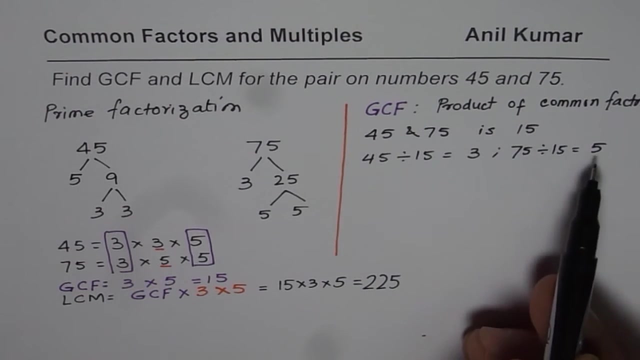 see that we can divide both by 15, right. 45 divided by 15 is 3, correct. And 75 divided by 15 is 5.. So you can divide both the numbers by 15 without any remainder right. 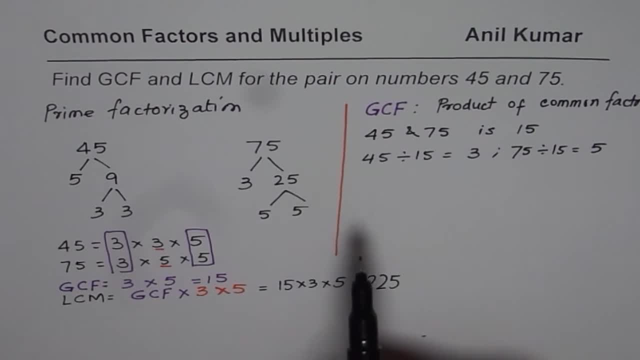 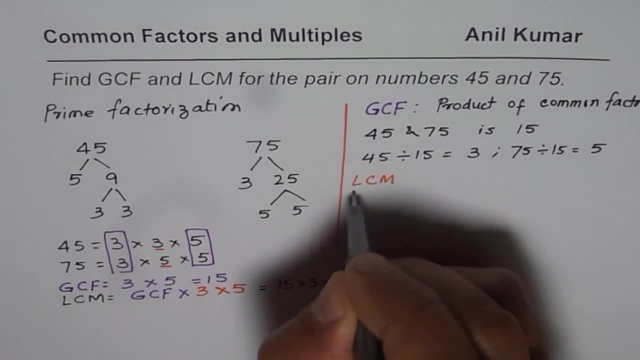 That is how we can find greatest common factor and that is the application. Now to find the least common multiple. what do we do? Least common multiple is the number which is smallest and which can be multiple of both right. So that is how we find least common multiple. You could. 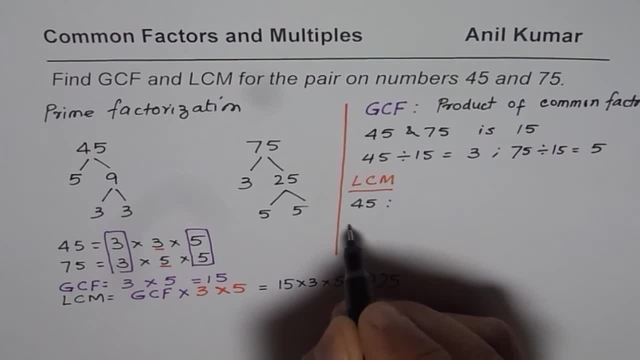 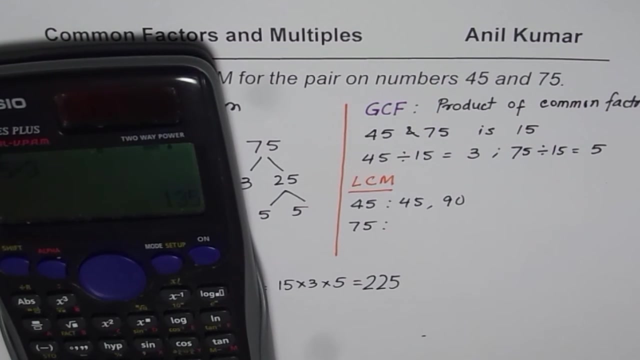 check. Let us write down multiples of 45 and 75, correct. So multiples of 45 will be 45 times 2, 90.. Let us use calculator. Keep on writing multiples of 45.. Times 3, 135.. So 45 times 4, 180.. 45 times 5, 225, and so on. Similarly, 75 multiples. 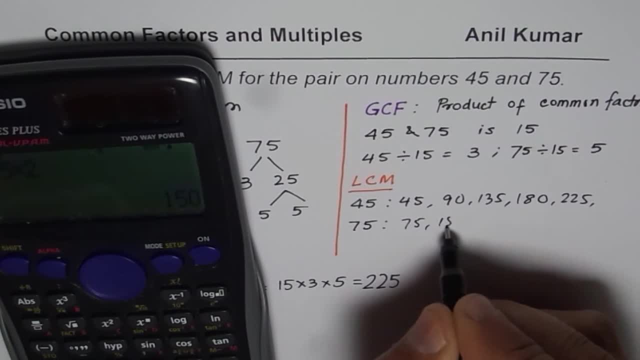 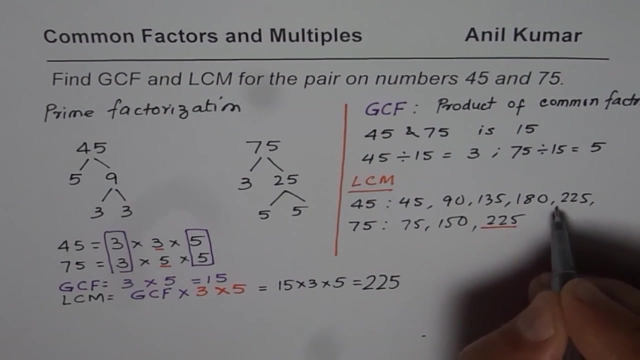 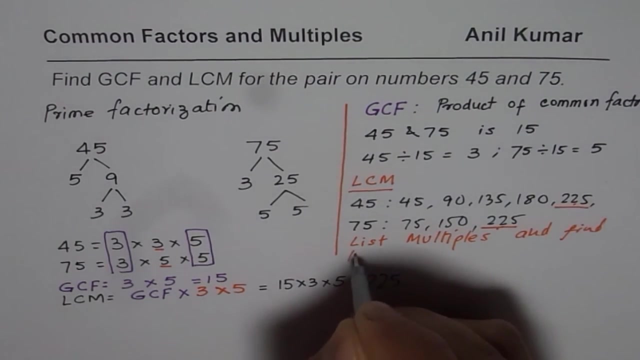 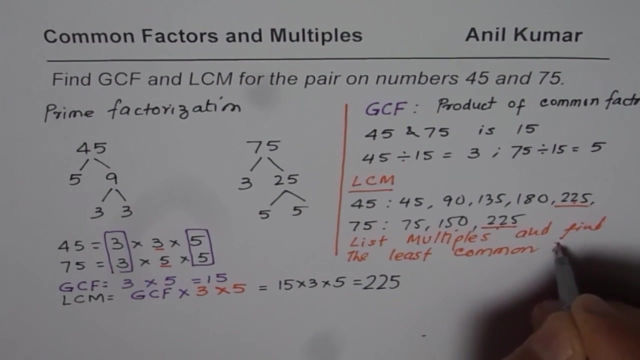 is fine, Of course. first is 75,, then 150, and then 75 times 3,, 225.. So in this list of multiples you find 225 to be the least common multiple, right? So this is another way to find least common multiple, that is, list multiples and find the least common in. 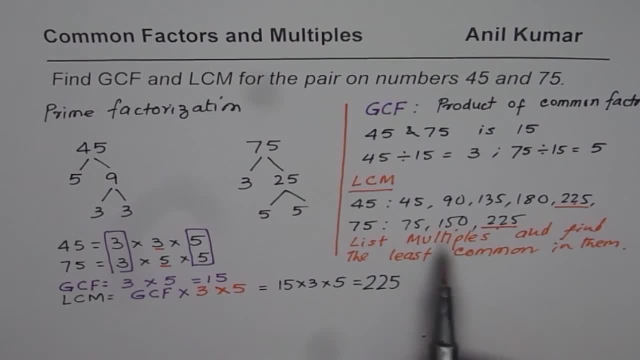 them right. So that is by definition. So you just write down the multiples, select the least common To get the answer. So we get the same answer as 225.. So that is an alternate method which I have discussed with you. but you could do with prime factorization also. So here we. 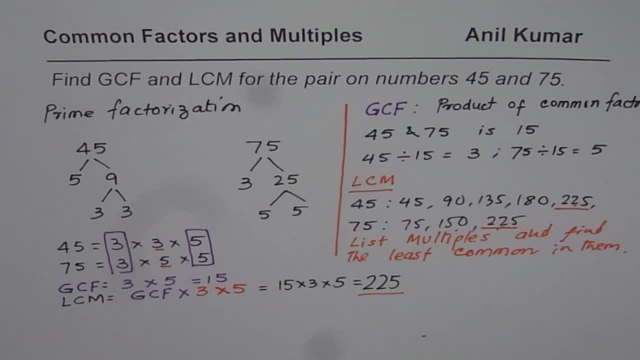 have two different methods to find LCM. I hope that helps. Thank you and all the best.